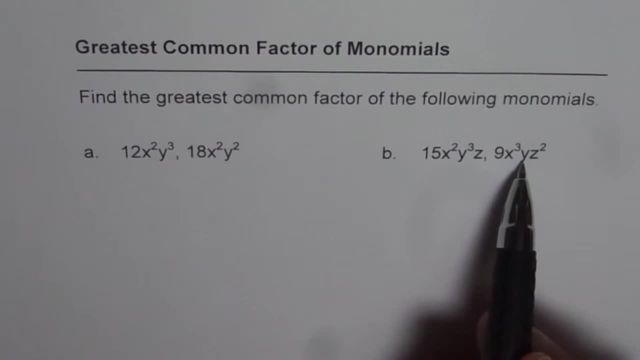 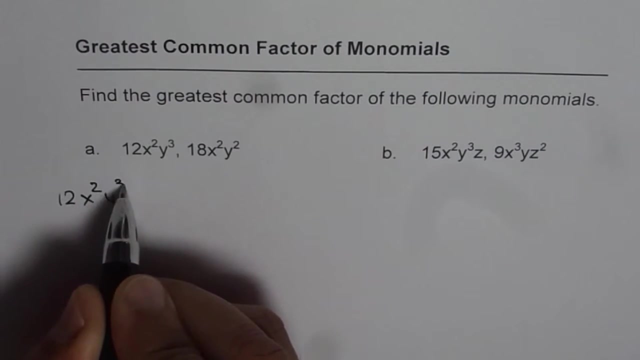 So let us start with the first one and find the common factors. Strategy to find common factors for monomials is similar to what we do in numbers, So let us begin with 12x square yq. We can write all factors of this monomial. 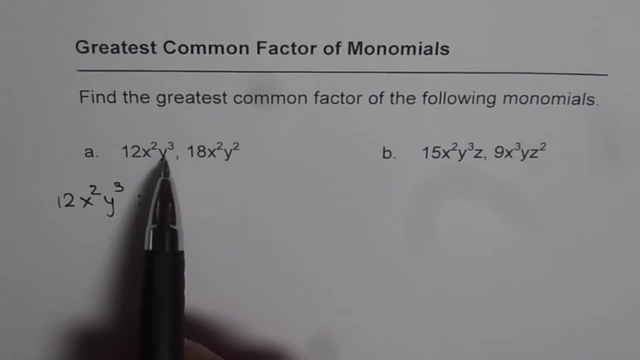 So monomial is a function of common factor. We can write all factors of this monomial. Lets begin with 12x. square yq is one of the monomials. We can write all factors of this. monomial has a constant term and the variable terms with exponents. Now the constant term is called the. 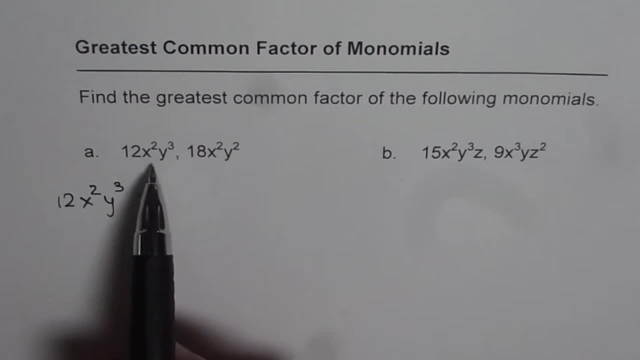 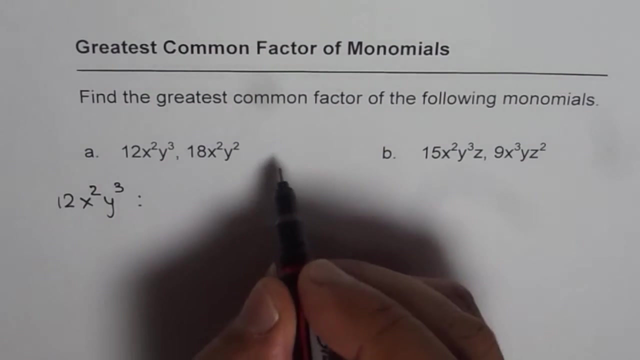 coefficient, as you know, and the variable terms are in this case x square and y cube. When we say x square, that means x times x, y cube means y times, y times y. So we have three factors of y, 2 of x, 12. we can write 12. with prime factorization We get. let's find prime factors of 12.. 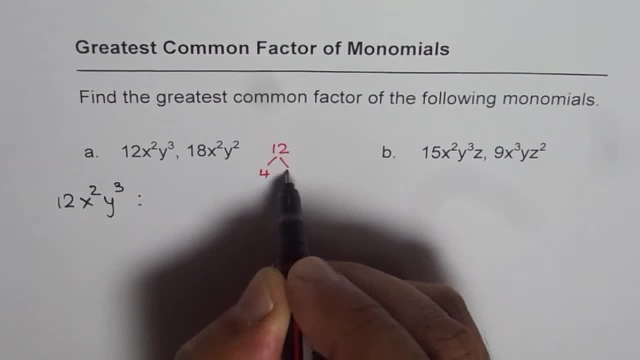 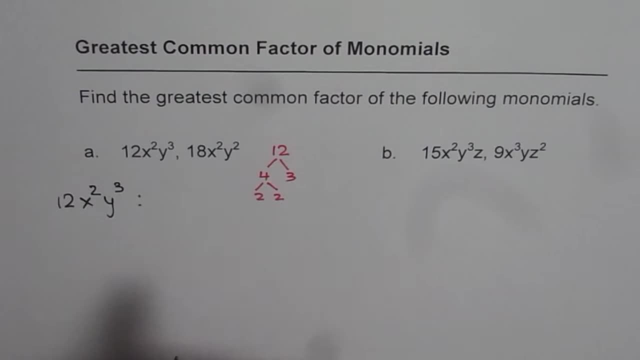 12 could be written as 4 times 3 and 4 could be written as 2 times 2, right? So we get prime factors of 12 as 2 times 2 times 3, correct? So let me write down all the factors of 12 x square. 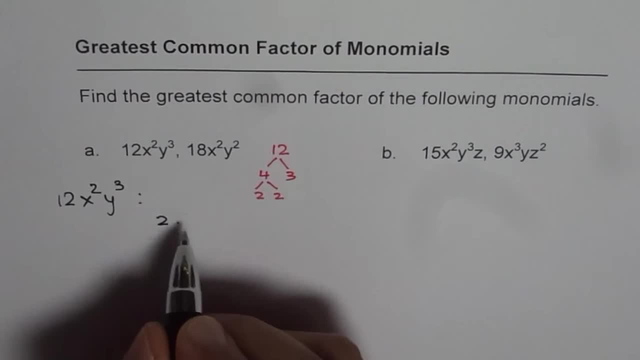 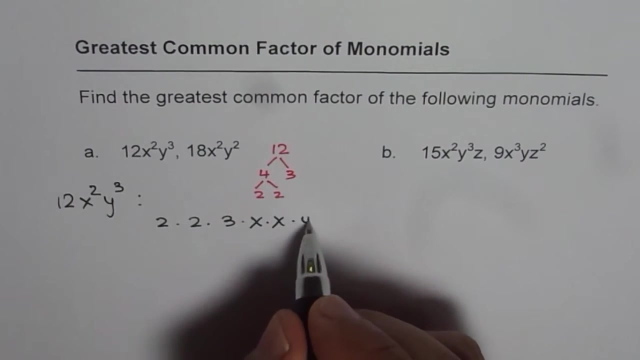 y cube. Let me write them here. So we get 2 times 2 times 3.. These are the prime factors of number 12, the coefficient of the first monomial. and then x square means x times x, y cube means y times, y times y. So that is how we can get. 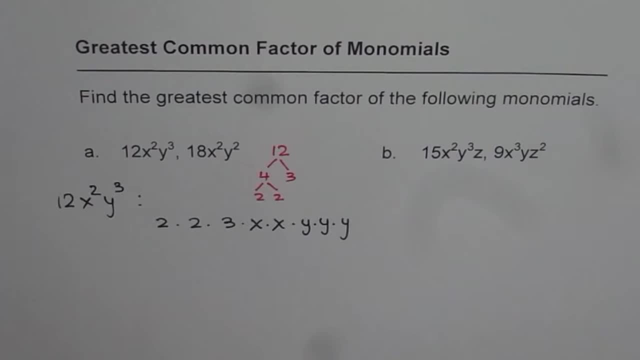 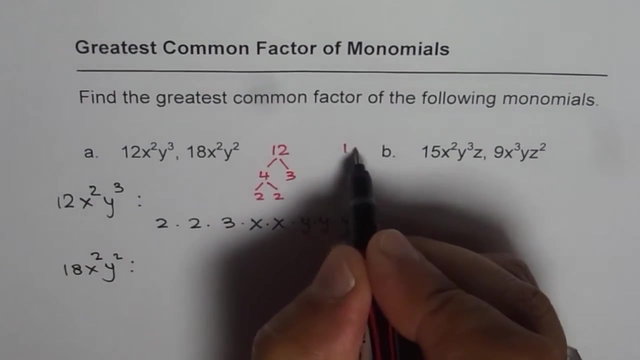 all the basic factors of the given monomial. Let's perform the similar operation on the second monomial, which is 1, 18, x square, y square. Now for 18, let's do the prime factorization: 18. you could write this as: 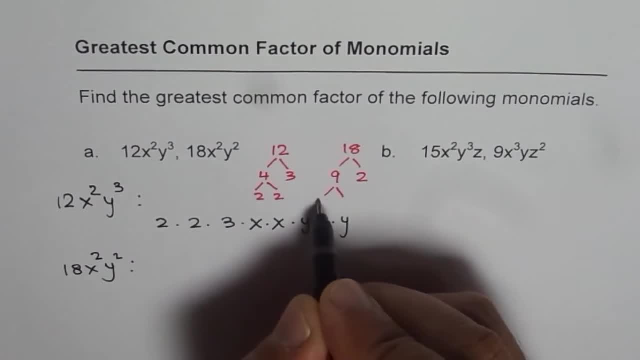 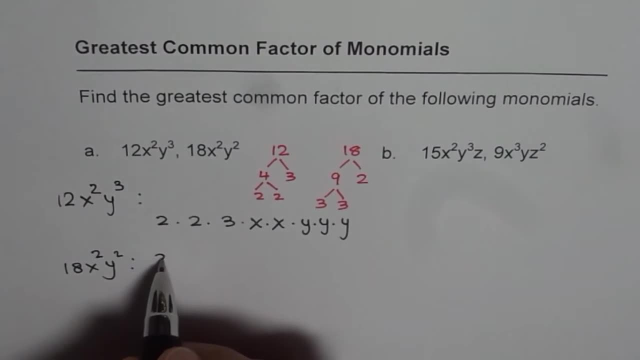 9 times 2 is 18 and 9 is 3 times 3, right? So that gives us all the prime factors for 18, which are 2 times 3 times 3.. x square means x times x. y square means y times x. So we get.